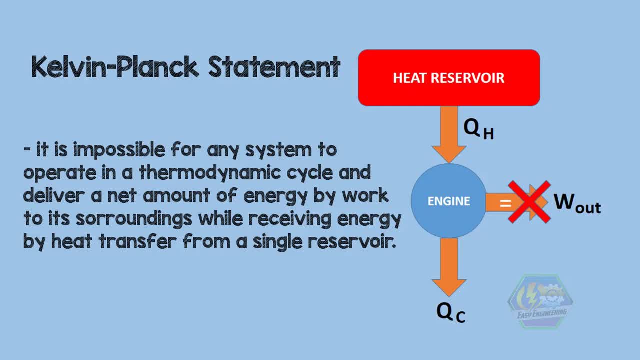 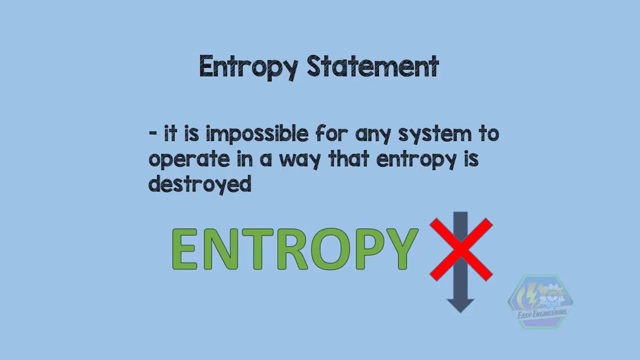 statement: it is impossible for any system to operate in a thermodynamic cycle and deliver an innate amount of energy by work to its surroundings while receiving energy by heat transfer from a single reservoir. Third statement is the entropy statement. it is impossible for any system to operate 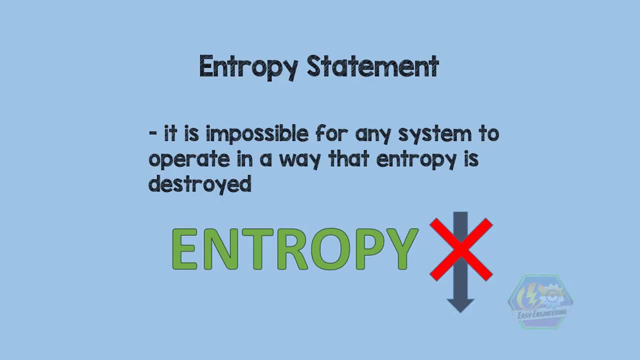 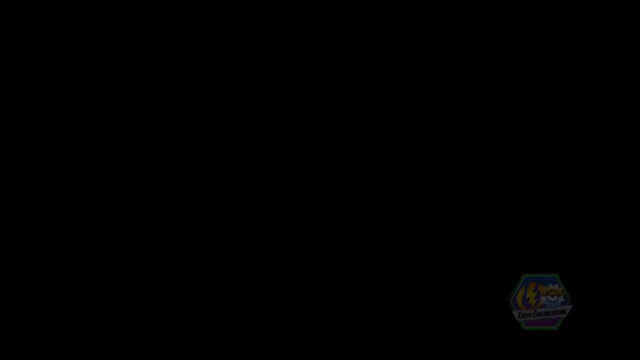 in a way that entropy is destroyed. So to make it easy, we made two easier statements that would help us more in understanding this law. So first is: well, let's call this as high to low. For any process, a natural flow will. 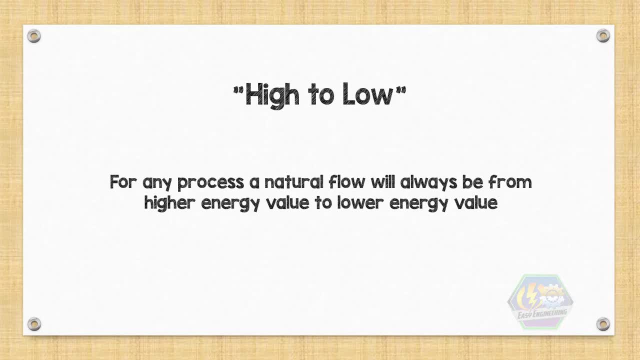 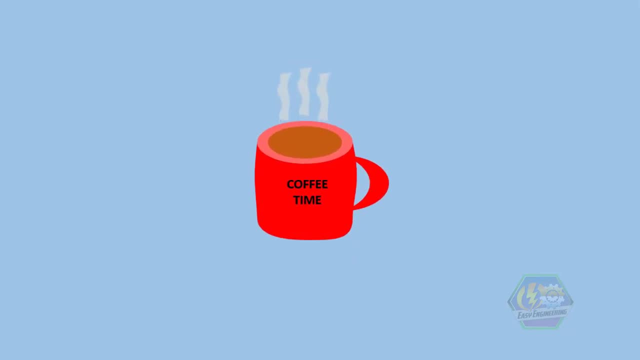 always be from higher energy value to lower energy value. For example, coffee. The temperature of coffee is higher than its cup, and that's what it says from higher energy value. So the temperature of coffee gets transferred to the cup, which is cooler, lower energy value. 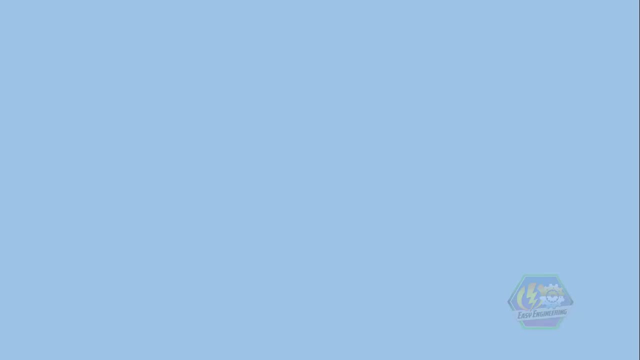 And that's why the cup gets hotter. Or try a compressed gas in a balloon. If you open a small hole in a balloon, does the outside air enters the balloon? No, instead, the gas in the balloon goes outside, transfers its pressure to the outside air, because the gas 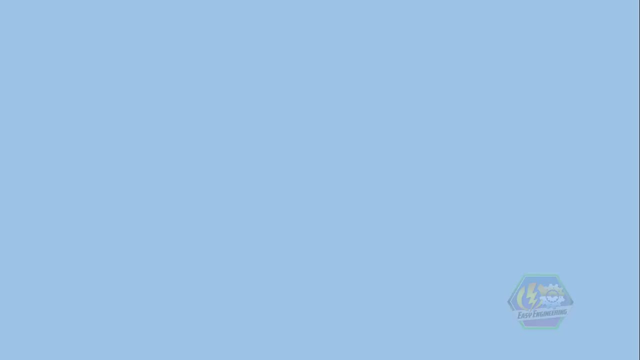 in the balloon has higher pressure than the outside air. Now let's look at another example. Let's say you have a professor connected to an empty tank with a valve in the middle. Now open the valve and what happens? The full tank level is lowered, transferring its level to the empty tank. 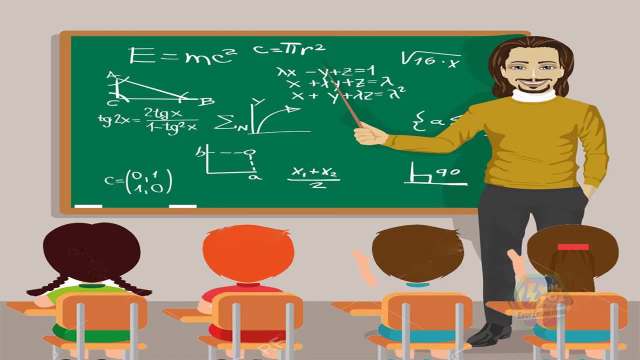 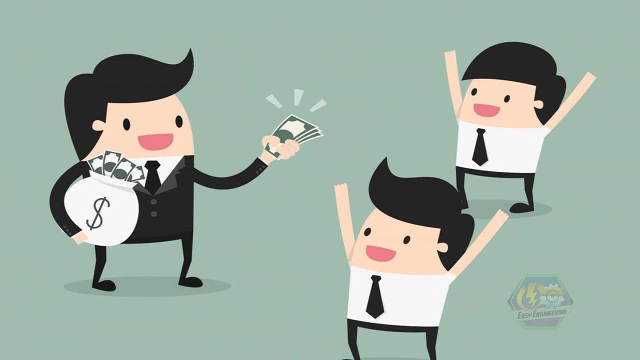 How about the topics being discussed in your classroom, That transfer of ideas comes from the professor, which has more ideas, to its students, which has lower ideas. Or even think of the salary from employer to employee. True, right. So now let's move to the second one. 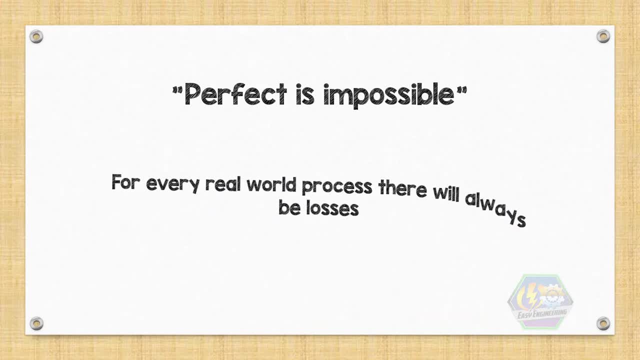 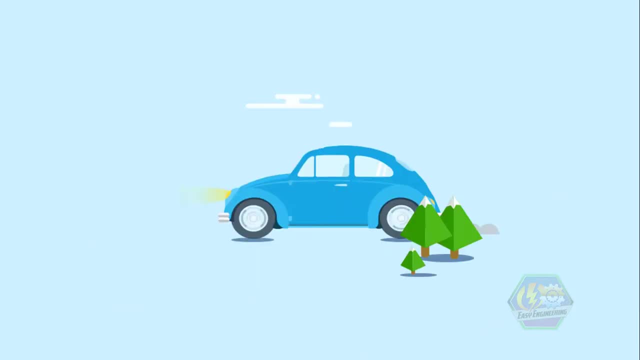 Let's call this. as For every real-world process, there will always be losses. That means you cannot convert all of your car's fuel into mechanical energy which can rotate your car's wheels Proof. It's the gases you see on the car's muffler. 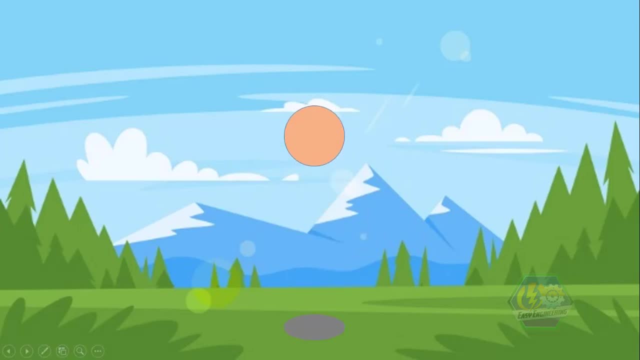 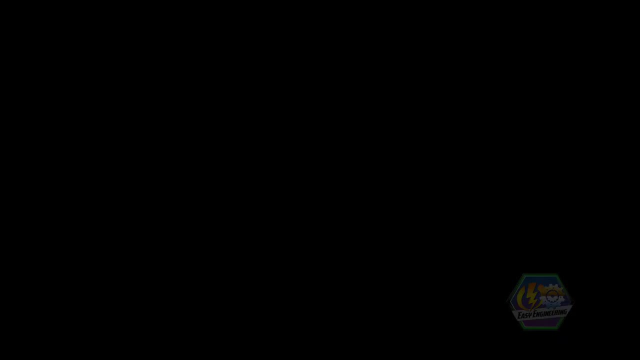 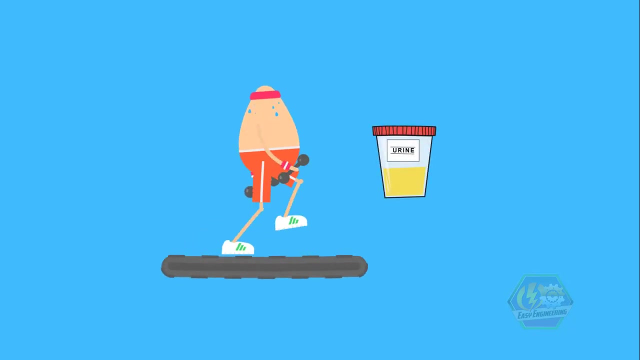 Or try bouncing a ball by first throwing it up to the air. See that as the number of bounces increases, the level of bounce decreases because of the loss of energy which is transferred to the ground. How about our foods? That is our source of energy. We can see the losses through our sweat, urine and solid.